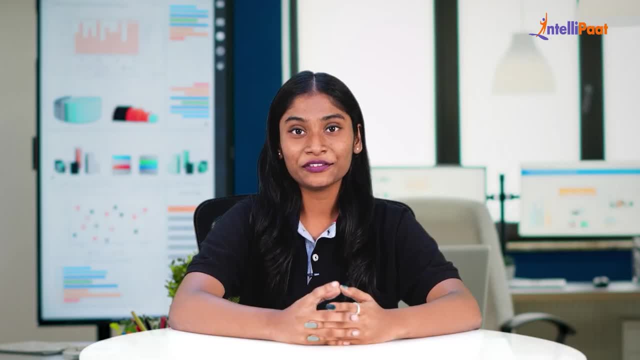 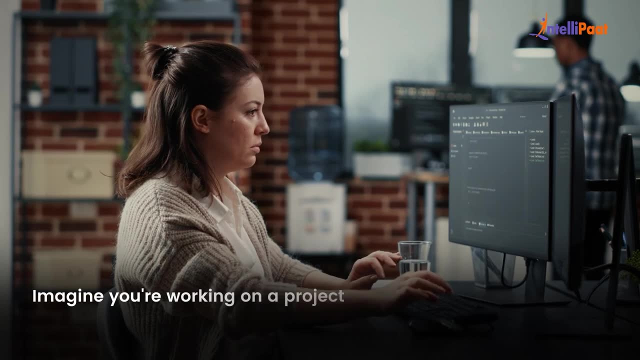 Hello everyone and welcome to this video by Intellipaat. In this video, we'll take a look at what is version control. Imagine you're working on a project, whether writing a code, creating a document or designing a website. Now, if you could turn back time and revisit. 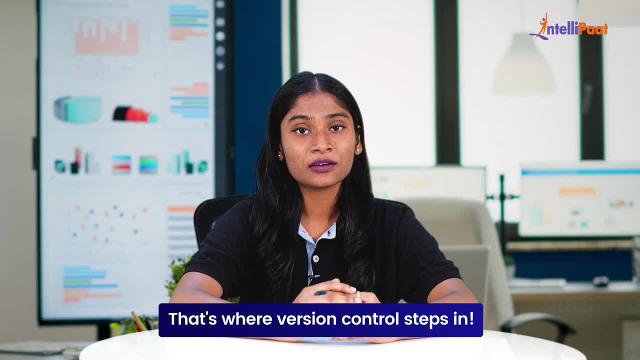 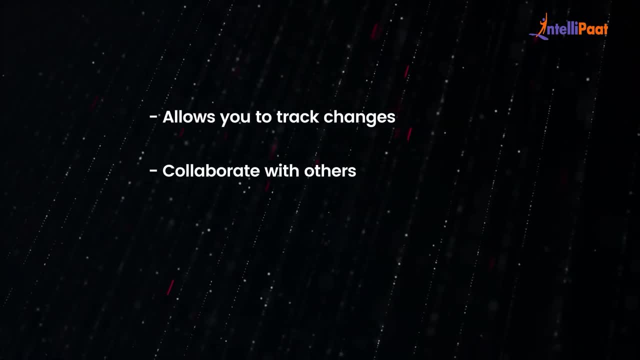 the previous version of your work. that's where version control steps in. Version control is like having a time machine for your project. It's a powerful system that allows you to track changes, collaborate with others and maintain the history of every modification made to your file. With version control, you can effortlessly switch between different 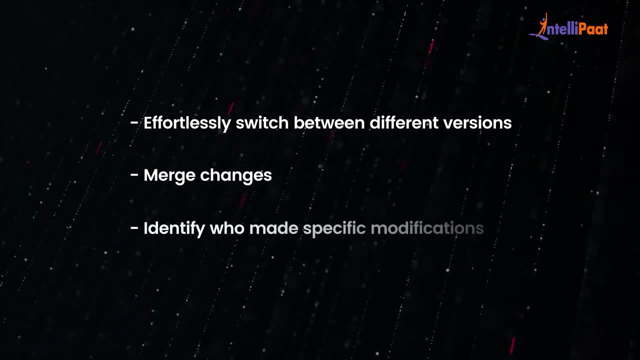 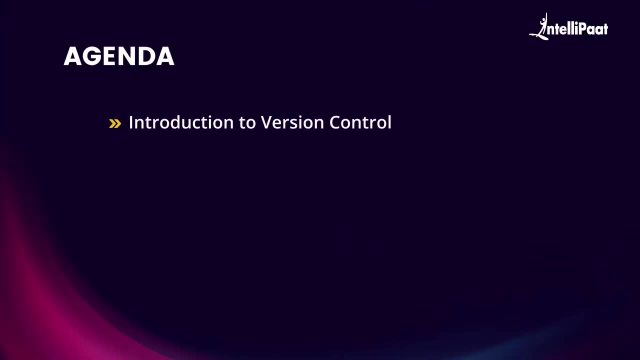 versions, merge changes and even identify who made the specific modification. Now let's take a look at our agenda. We would start our video with introduction to version control and then we'd see some of the basic concepts in version control. And once done with that, 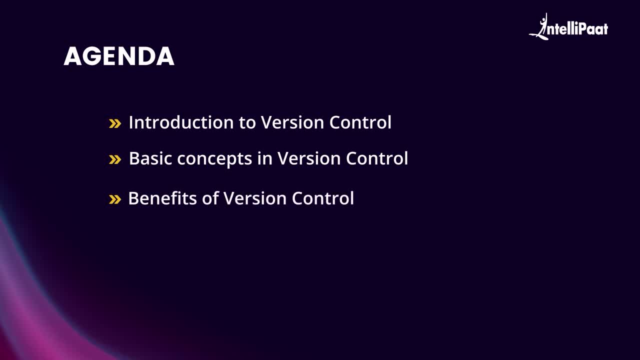 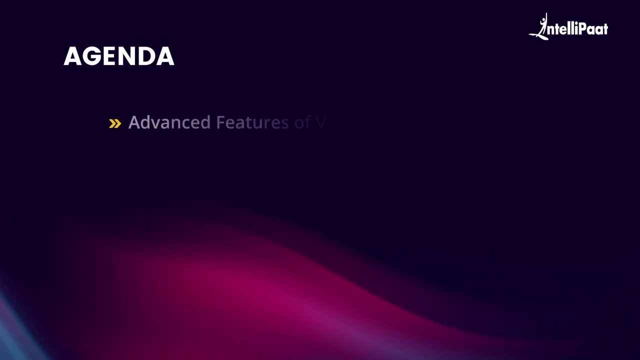 we would be exploring the benefits of version control and then learn the version control system. Later we would dive into the basics of version control. and then we would explore the benefits of version control and then learn the version control system. Later we would dive into the workflow and collaboration in version control and we would see the advanced features. 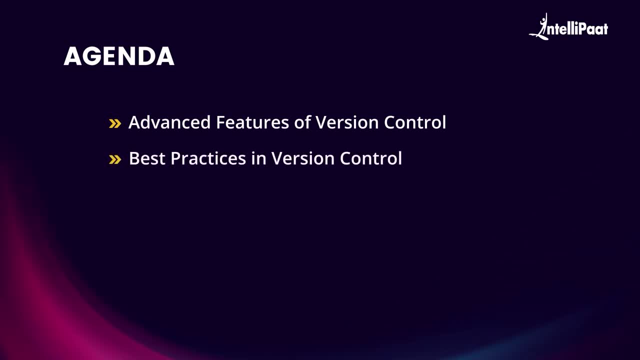 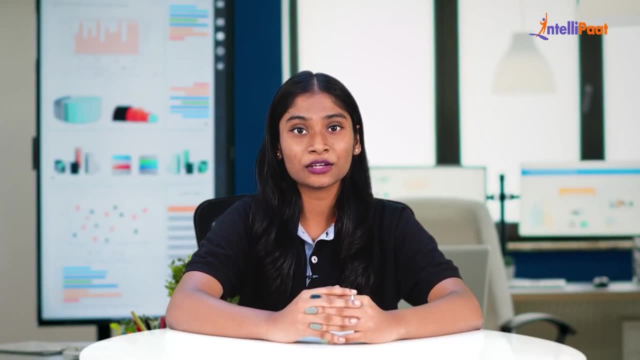 of version control and the best practices in version control, And we would be summing up our video with a conclusion. So buckle up and get ready to dive into the exciting journey of managing your project's evolution, But before that, please make sure you subscribe. 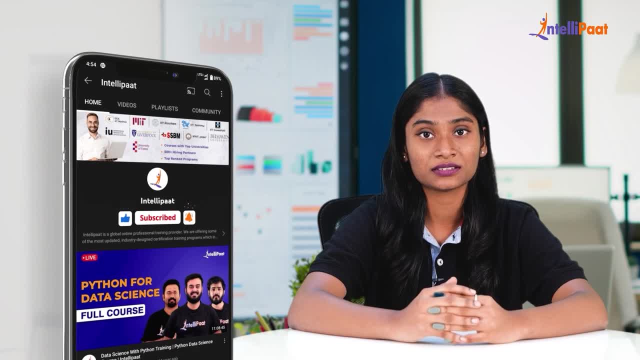 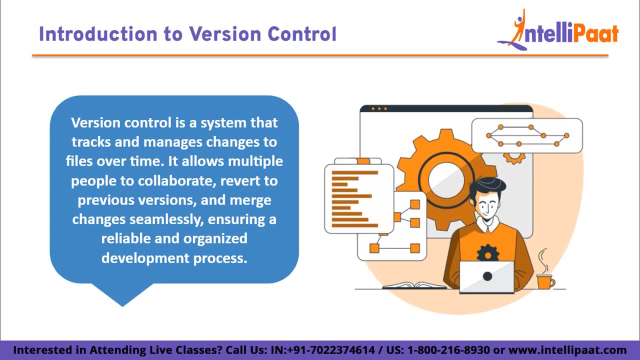 to our YouTube channel and hit the bell icon for regular updates from us. Now let's start with our first agenda: introduction to version control. In the world of collaborative project, version control is a powerful tool that helps you to manage and track changes in your file over time. It acts as a safety net, allowing you to go back in time and access. 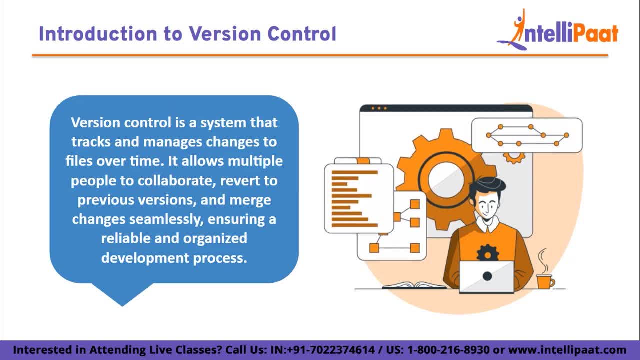 the previous version of your work. Imagine you are working on a document with a team and everyone is making edits simultaneously. With version control, you can keep track of who is making what changes, merge those changes together seamlessly and easily revert to an earlier version if needed. Let us consider an example using a software development. Let 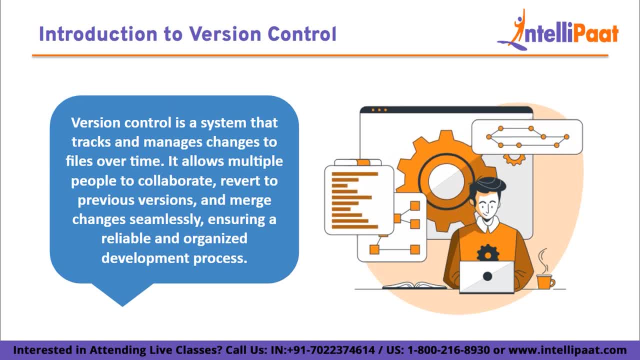 us say you are working on a program with multiple developers. Version control enables the developers to work on their own copies of projects while maintaining a central repository that helps you to maintain versions. Whenever someone makes a changes, they create a commit which captures a snapshot of the file. at the moment, These commits are organized in a timeline. 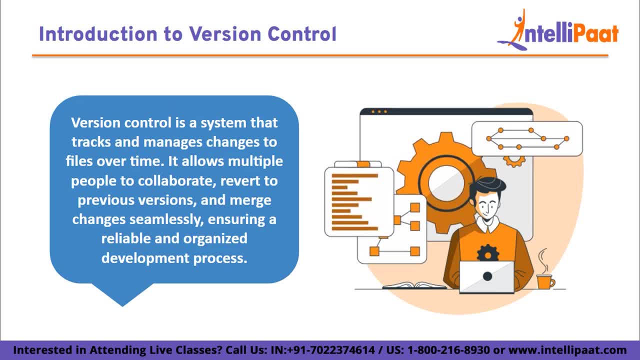 allowing you to see the progression of the file and compare the different versions. Version control systems like Git are widely used to manage and track changes in your project. They are widely used and offer powerful features. They allow you to create branches which are like separate paths of development. For example, you can create a branch to work on a new feature. 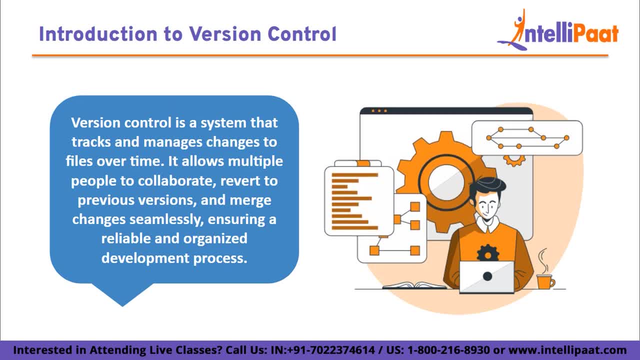 without disturbing the main codebase. Once the feature is complete, you can merge it back into the main version In the nutshell. version control keeps your project organized, making the collaboration smooth, and provides safety net for changes. It's like the time machine for your file, ensuring that you can always access the previous version of your 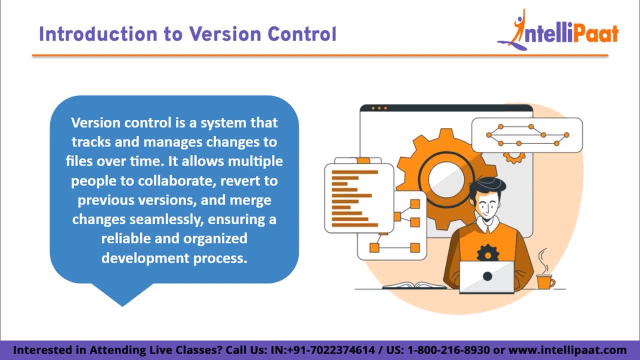 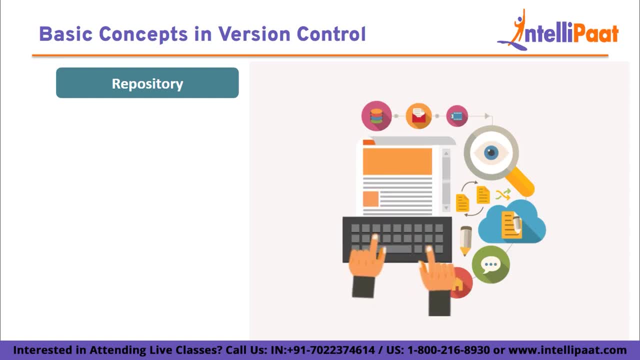 project. Now let's see some of the basic concepts of version control. Repository- A repository is a central storage location where all the files and the versions are stored. It serves as a database that maintains the complete history of changes made to the project Commit- A commit is a snapshot of the changes made. 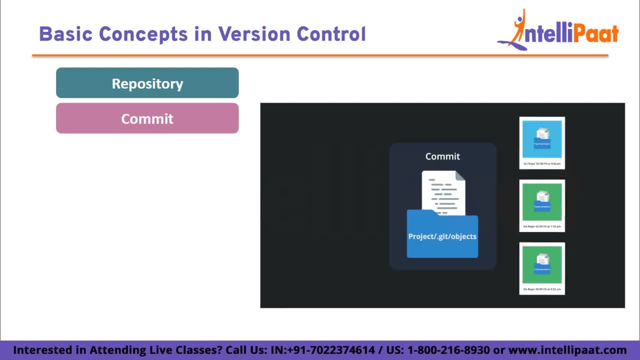 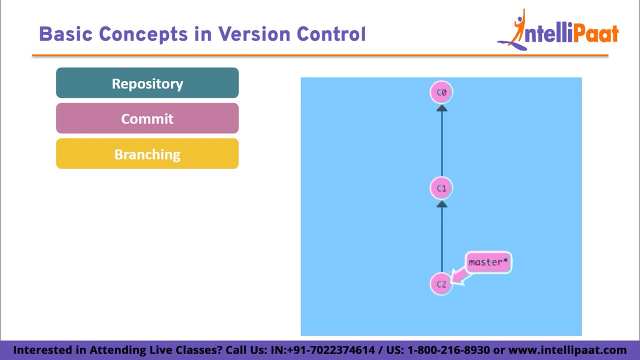 to one or more files at the simultaneous point of time. It captures the modification, addition or deletion and includes the metadata such as author's name, timestamp or a descriptive message Branching. Branching allows the creation of separate lines of development within a project. It enables the parallel work on different features or 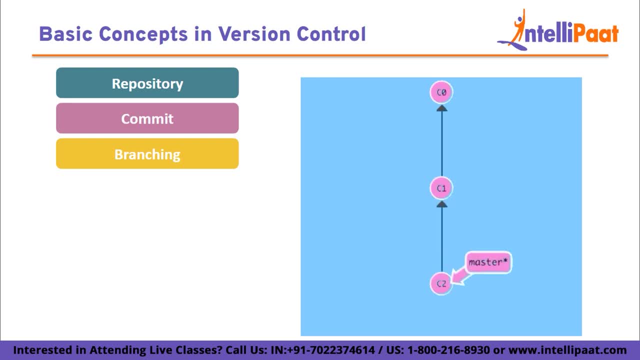 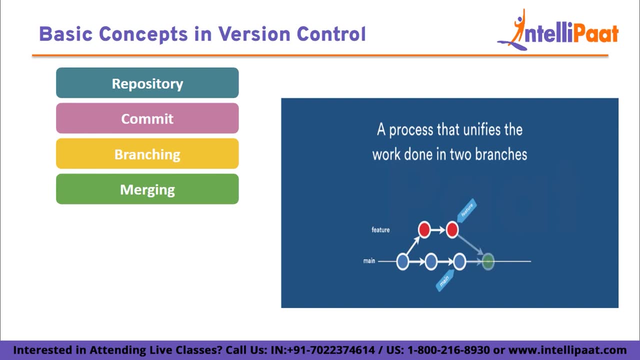 bug fixing independent of the main code. Branches can be created, merged or deleted as needed. Merging: Merging combines changes from one branch into another. When work on a branch is complete, the changes can be created and deleted. The changes can be integrated back into the main code or another target branch, ensuring the 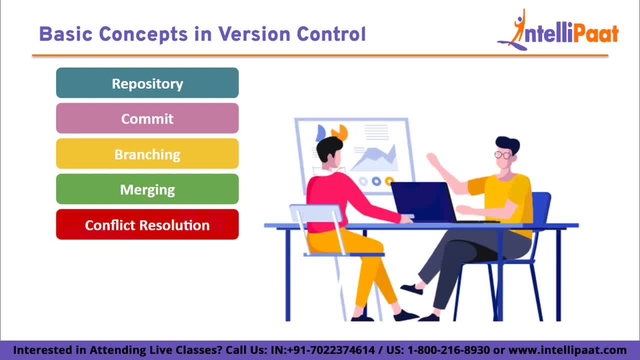 cohesive and an up-to-date project. Conflict Resolution: Conflict resolution occurs when multiple changes conflict with each other, such as two developers modify the same line of code. Version Control System provides mechanism to identify and re-solve the conflict during the merging process. History and Tracking Version Control System maintains a detailed 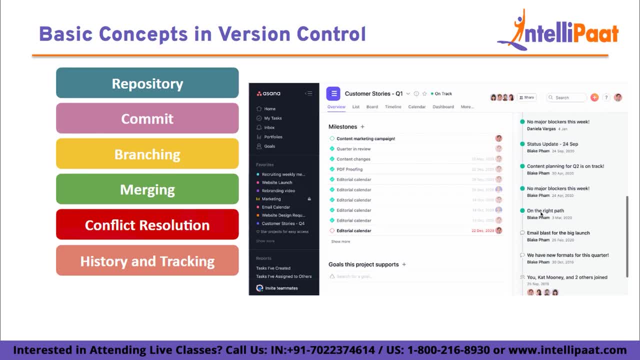 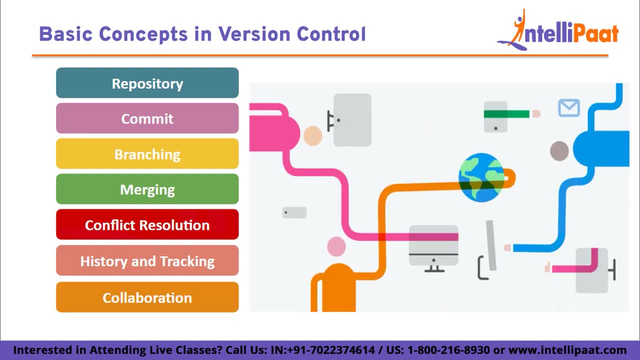 history of all the changes made to the project. This allows you to track the evolution of file, review previous version and understand who made the changes and when. Collaboration: Version control facilitates collaboration amongst the team members. Multiple developers can work on the same project simultaneously. 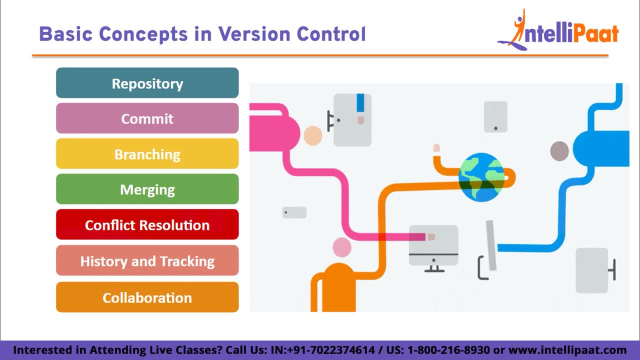 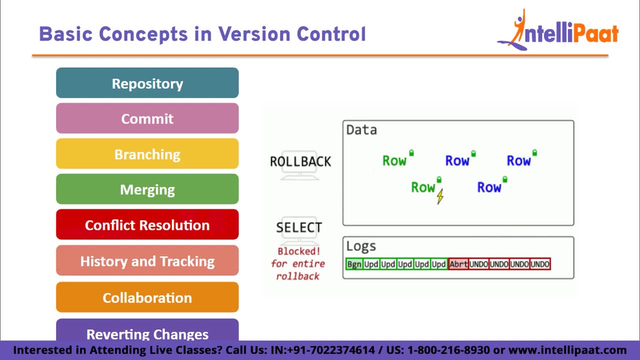 with an ability to share and synchronize the changes seamlessly. Reverting Changes- Version control enables you to roll back to the previous state of your project. If a mistake is made or an understatement is made, you can easily revert to a previous commit to ensure the project stability. 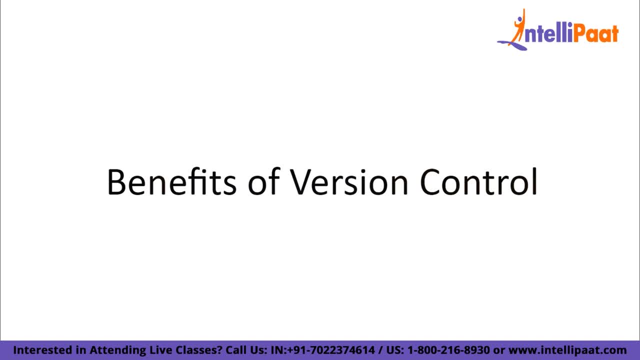 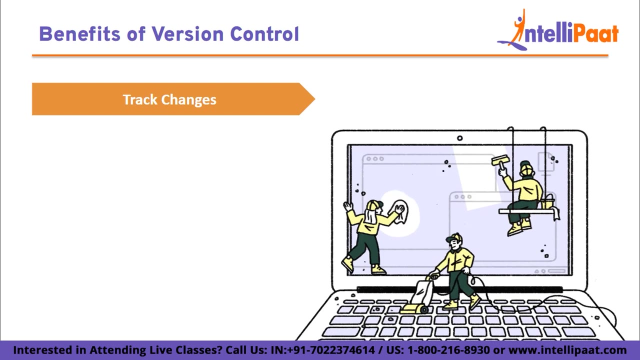 Version Control brings numerous benefits to the table: simplifying project management, enhancing collaboration and providing safety net for development. Key benefits of version control: Track changes. Version Control allows you to track and document every modification made to your project. You can easily see what changes were made when. 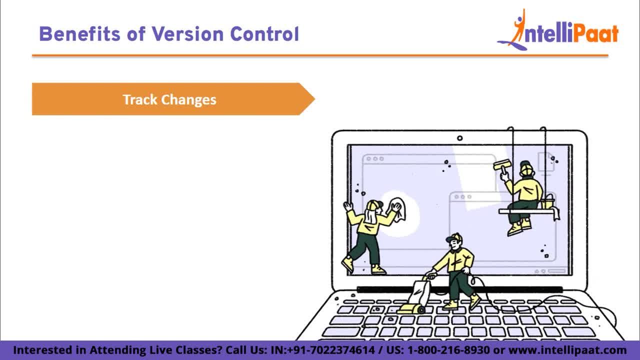 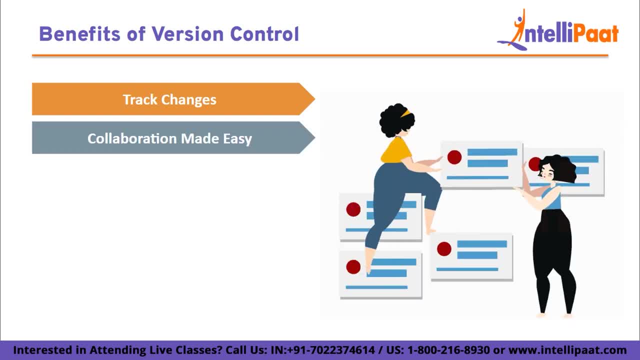 they occurred and when they will not be made. You can easily see the rest of all the changes and who made them. This visibility helps you to understand the project's evolution and facilitate troubleshooting and debugging. Collaboration made easy. Version control enables seamless collaboration amongst the team members. Multiple people can work on the same project. 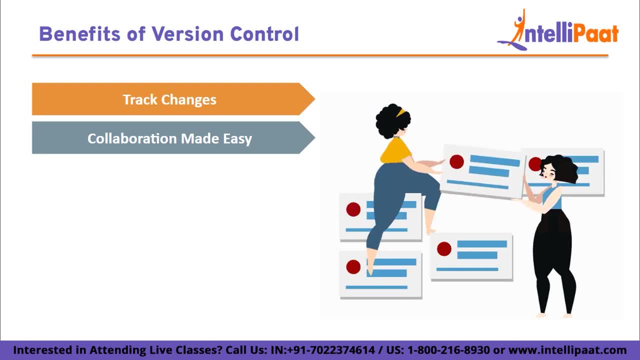 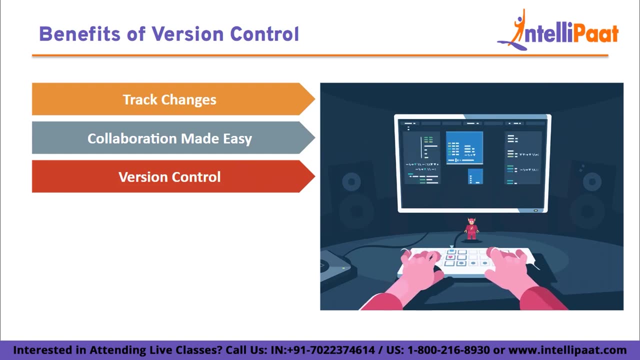 simultaneously, each with their own copy. Version control system provides efficient mechanism to merge and synchronize changes made by different contributors, ensuring a smooth collaboration process. Version control: With version control, you have a complete history of the project version. You can access any previous date or iteration of your project, allowing you to compare different. 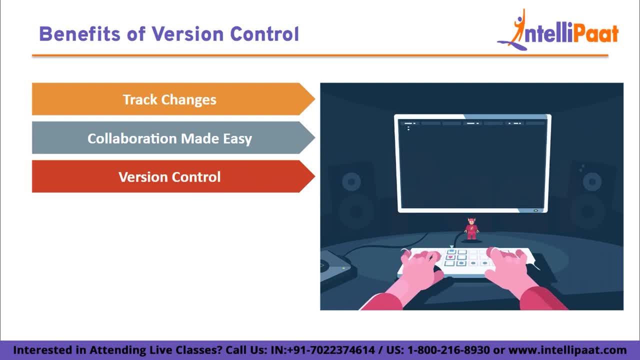 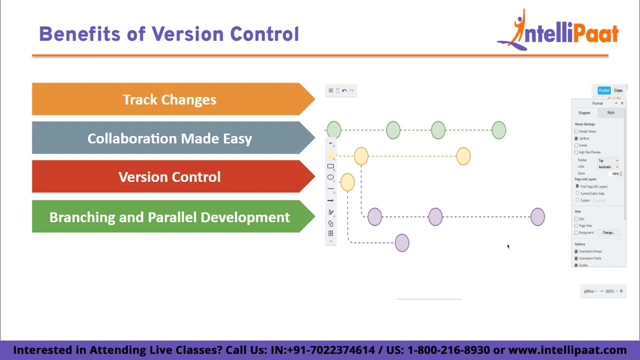 versions roll back to the earlier version or recover the lost work. This capability provides the safety net enabling you to experiment with new ideas without fear of irreversible consequences. Branching and parallel development: Version control system allows you to create branching and parallel development. This allows you to create branching and parallel. 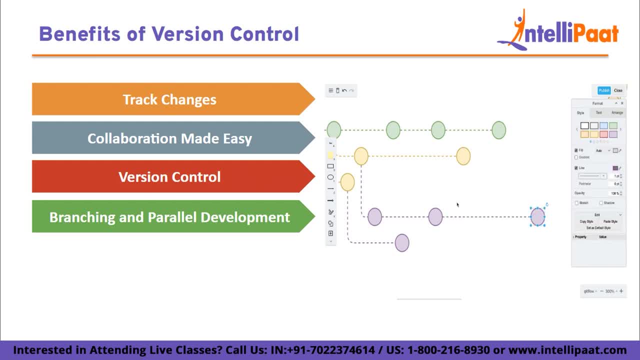 development. This allows you to create branches which are independent lines of development. This feature enables you to work on different features, bug fixing or experiment in separate branches without affecting the main code. Branches provide isolation and flexibility, and once a branch is ready, it can be merged back into the main project. 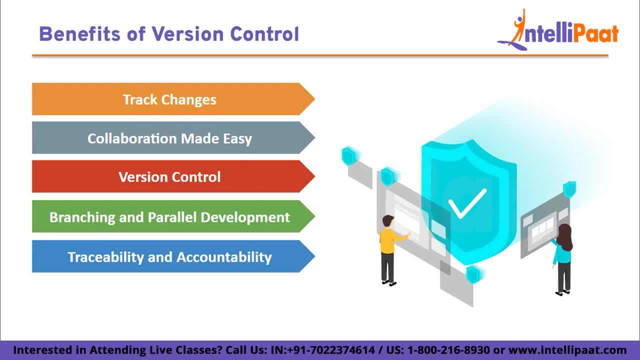 Traceability and accountability. Version control provides traceability by associating each changes with the author, timestamp and relevant information. This helps you to understand who made specific modification and why. It also promotes accountability, as everyone's contribution are tracked and can be reviewed. Conflict resolution In collaborative project. 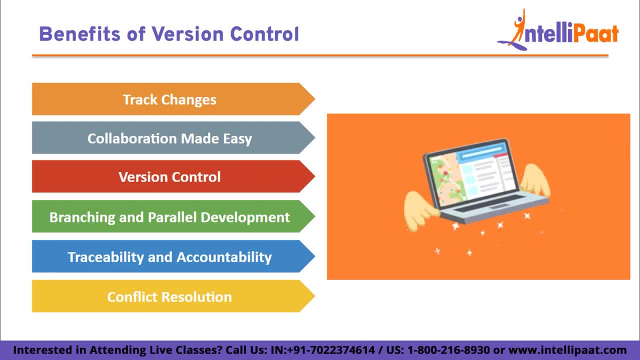 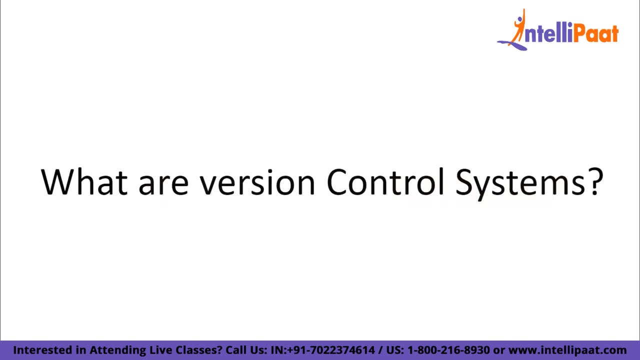 conflict may arise when multiple people modify the same file simultaneously. Version control system offers the tool to detect and manage this conflict, making it easier to resolve them and avoid the loss of valuable work. What are version control system? The version control system is a 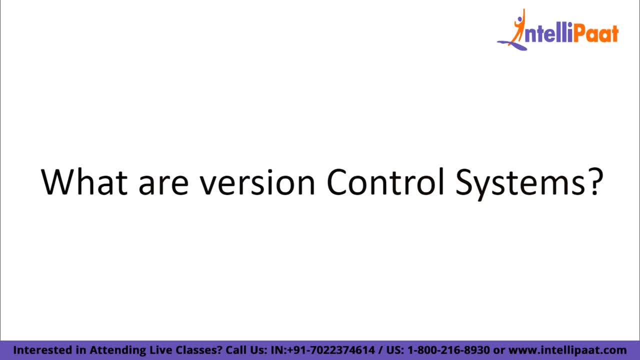 software tool that helps you to manage changes made to the file over time. It keeps track of all the modification, allows multiple people to work on the same project simultaneously and provides history of all the changes made. So here are a few important points of version control system. 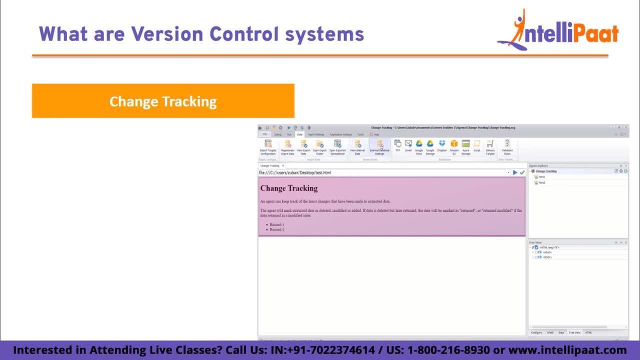 Change tracking: Version control system records changes made to the file, including addition, deletion and modification. It keeps a detailed log of all the changes made to the file. It also keeps a log of every modification, allowing you to see the complete history of the project. 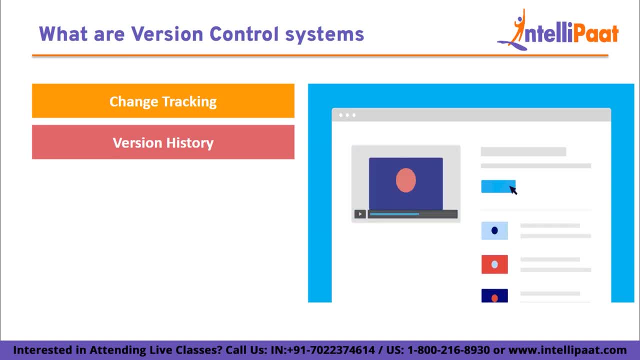 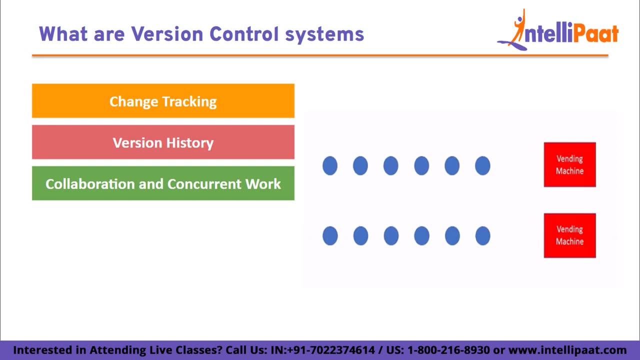 Version history: VCS maintains a chronological record of all the version of files and the entire project. This history allows you to access and revert to any previous version, compare different versions and understand how the project has evolved over time. Collaboration and concurrent work: VCS enables multiple users to work on the same project simultaneously without conflict. 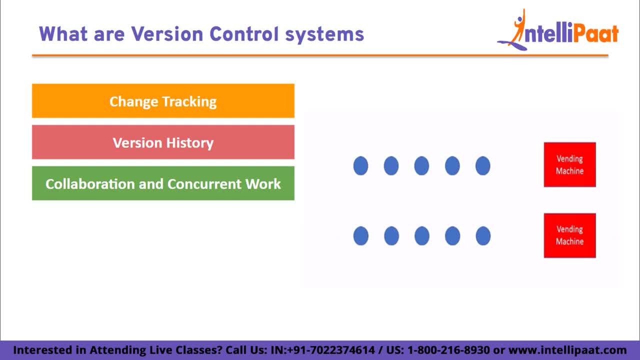 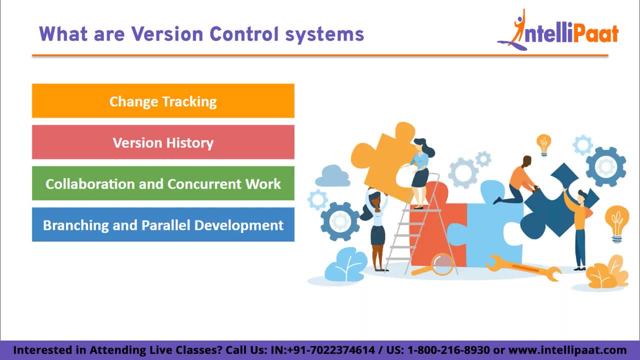 It provides mechanism to merge changes over the different users, ensuring smooth collaboration and preventing data loss or overwriting. Branching and parallel development: VCS allows for creation of branches, which is independent line of development. Branches enable the isolation of features or experiment, facilitating parallel work. 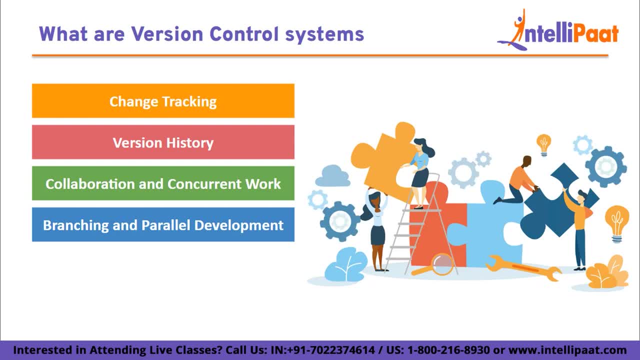 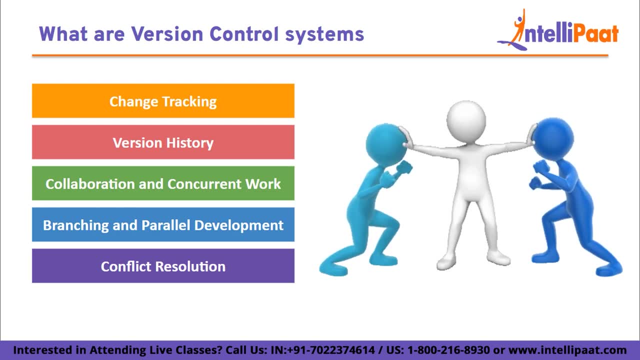 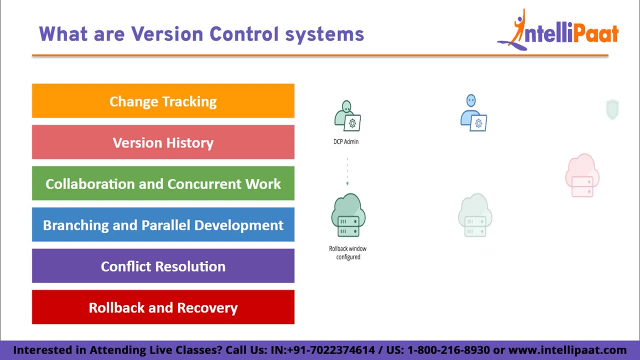 and allows changes to be made back into the main project when ready. Conflict resolution In collaborative environment, conflicts may occur when multiple users modify the same file simultaneously. Roll back and recovery VCS allows you to easily revert to the previous version or undo specific changes if needed. This feature provides a safety net. 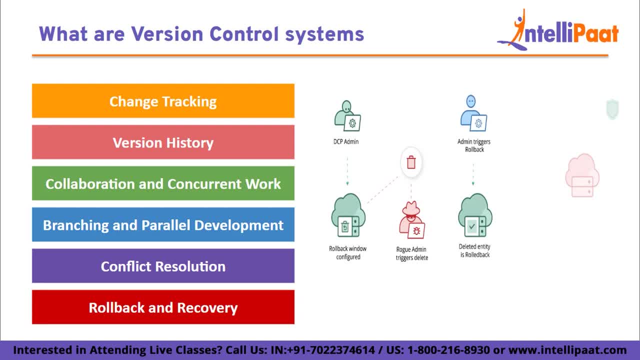 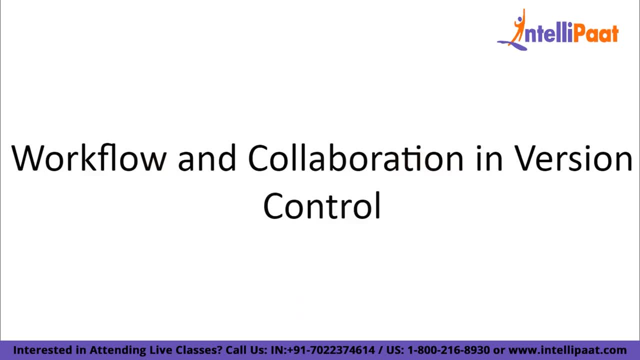 allowing you to recover from mistakes, experiment without fear and maintain the project stability. Workflow and collaboration are essential components of Version Control System. They play a crucial- a crucial role in enabling team to work together efficiently and seamlessly. Here's a closer look at the workflow and collaboration in version control. 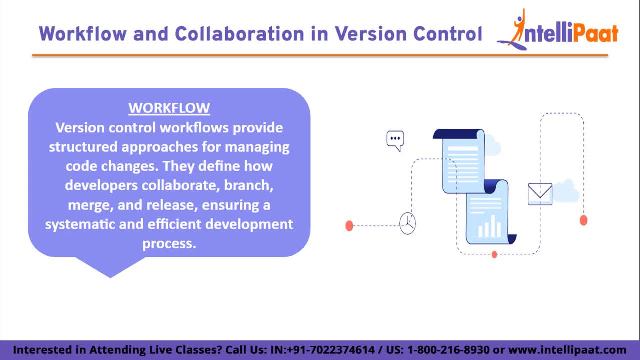 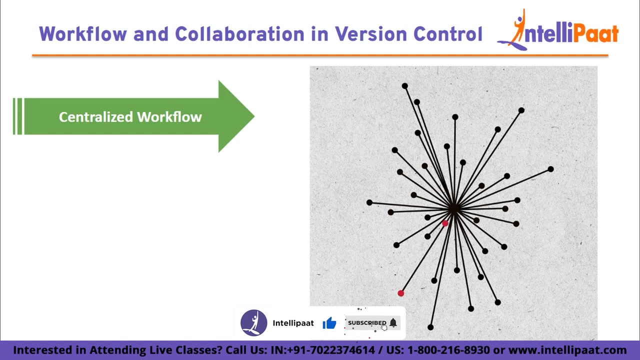 Workflow. A workflow in version control refers to a series of steps and processes following a team or an individual when working with version control file. Different workflows can be adopted based on the project requirement, team size and development practices. Some common workflow includes Centralized workflow. This workflow involves a central repository. 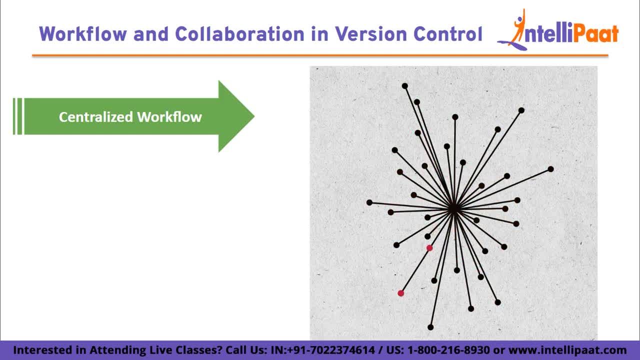 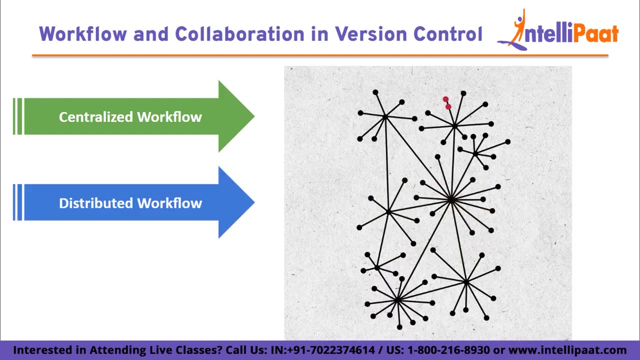 where all the developers commit the changes. It follows a linear structure where developers pull the latest changes from the central repository, making modifications and push the changes back. It provides a centralized and controlled approach to the collaboration Distributed workflow. In a distributed workflow, a team or a team of developers can work together to create. 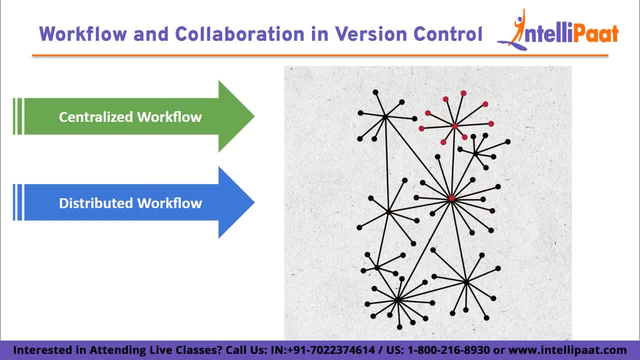 changes. Each team member has its own copy of repository. Development can commit changes locally and synchronize them with other repository. They allows for more independence and flexibility, enabling developers to work offline and merge changes at the later stage. Feature: branch workflow. The workflow involves creating separate branches. 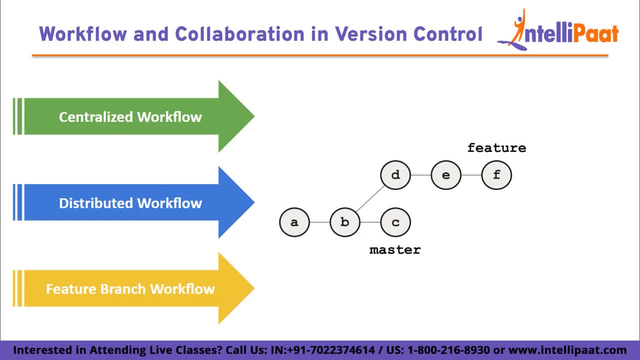 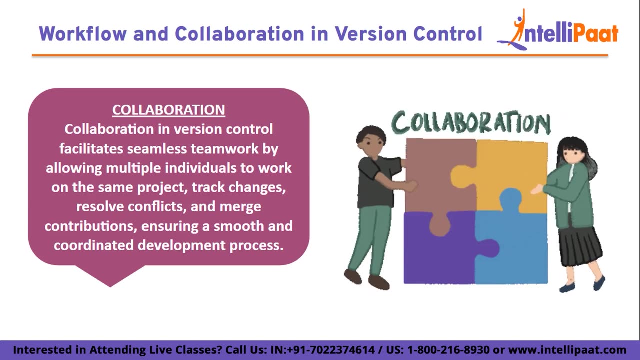 for the different features or tasks, Developers work on the respective branches, making changes and testing them independently. Once a feature is complete, it is merged back into the main branch. It enables parallel development and easy tracking of individual features. Collaboration- Version control provides collaboration features. 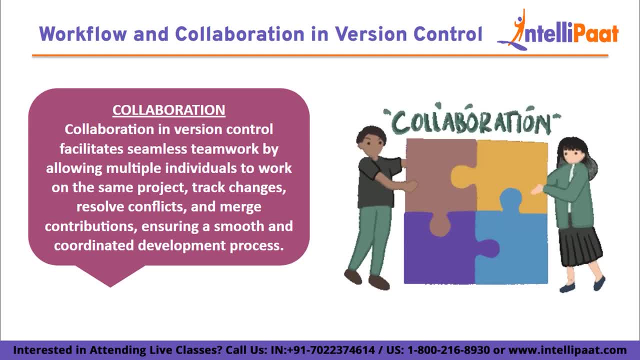 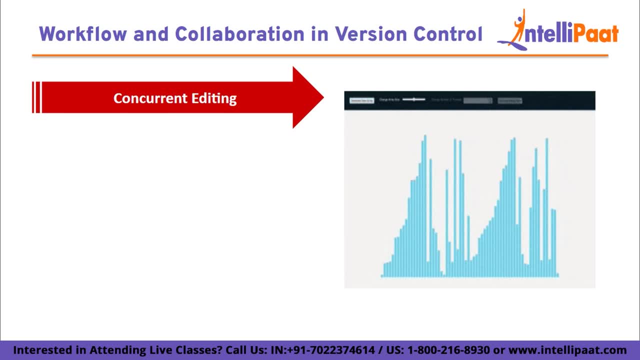 that enhance the team productivity and stream line development. These collaboration capabilities involve concurrent editing. Version control system allows multiple team members to work on the same file simultaneously without conflict. Each member can modify the files simultaneously, can modify the file independently and the system provides mechanism to merge and resolve. 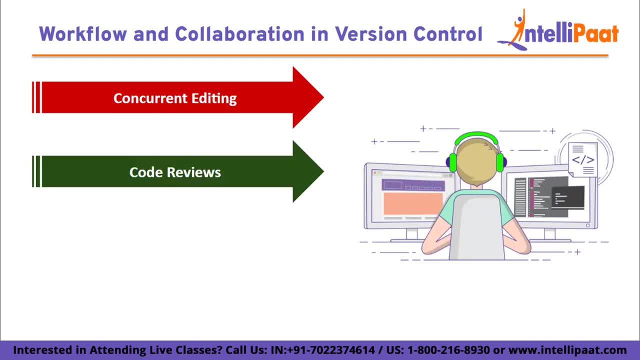 the conflict that arises. Code review version control system can integrate with the code review tools and provide the built-in review capability. This enables the team members to review and provide feedback on each other's changes, ensuring code quality, adhering the best practices and knowledge. 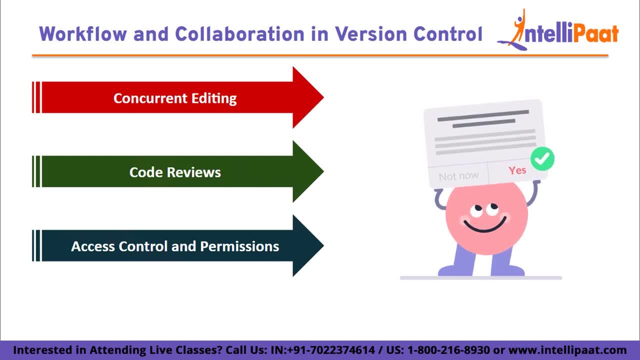 sharing within the team. Access control and permission. version control system allows the administrators to set the access control and permission. This ensures the team members to have an appropriate level of access to the repositories, branches and the file, safeguarding sensitive code and maintaining the data integrity. 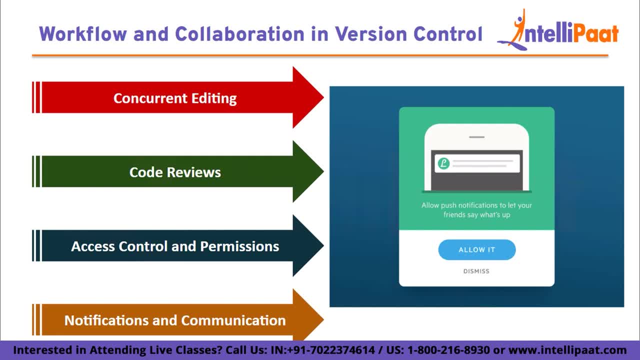 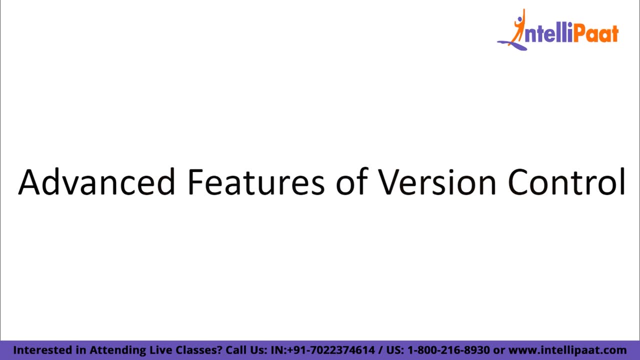 Notification and communication. version control system often provides notification mechanism to inform the team members of important events such as new comments, merge request or conflict. Advanced feature in version control system enhances productivity, flexibility and efficiency. They provide additional capability behind the basic functionality, allowing for more. 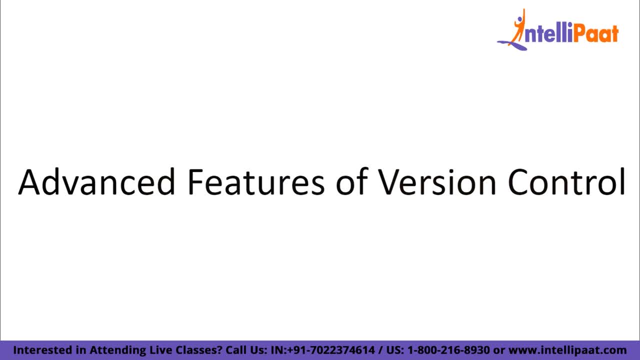 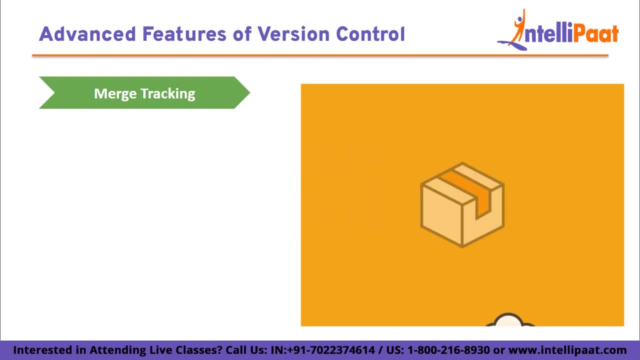 sophisticated version control workflow. So here are some of the notable advanced features: merge tracking: Merge tracking is a feature that helps in managing the complex merging scenario. It allows the system to keep track of which change set has been merged into the different branches, making it easier to identify. 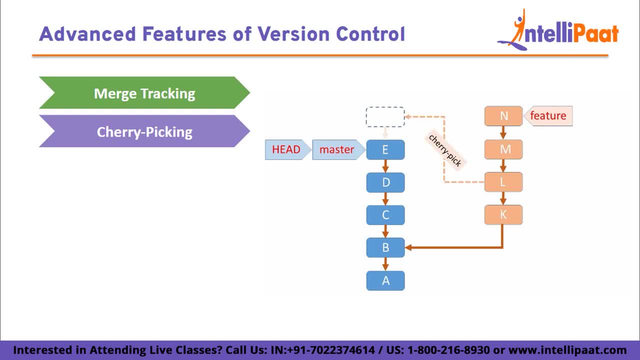 and handle the merge conflict. Cherry picking. cherry picking allows you to select specific changes from one branch and apply them to another branch. This feature is useful when you want to include specific changes or fix them from one branch to another without merging to the entire branch. 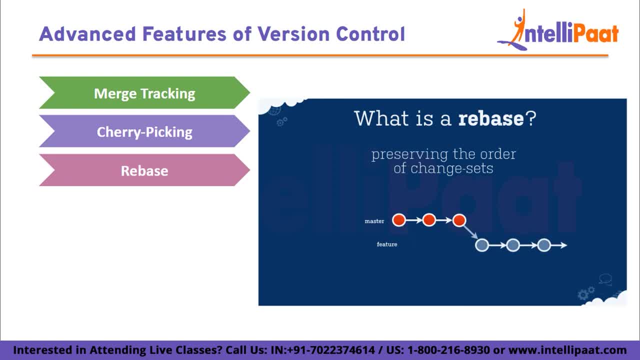 Rebase. rebase is a powerful feature that allows you to modify the history of branches. They allow you to move or integrate the commit from one branch to another, making it commit history clearer and more organized. Rebase can be used to modify the history of branches. 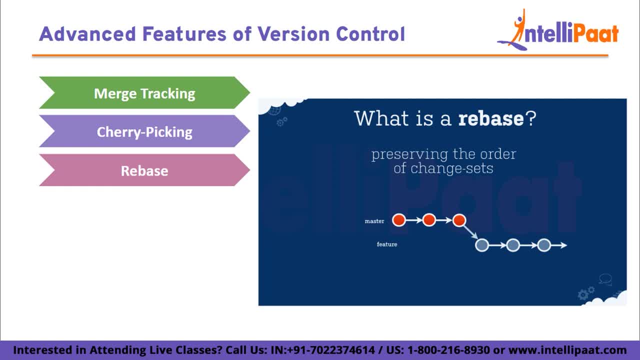 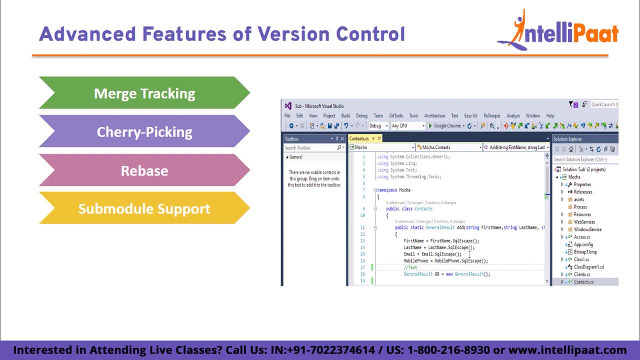 Rebase can be used to combine the commit, reorder them and apply them on the top of the latest changes. Submodule support: submodules enable the inclusion of external repository within the main repository. They allow you to manage dependency and incorporate external libraries, making it cheaper to work. 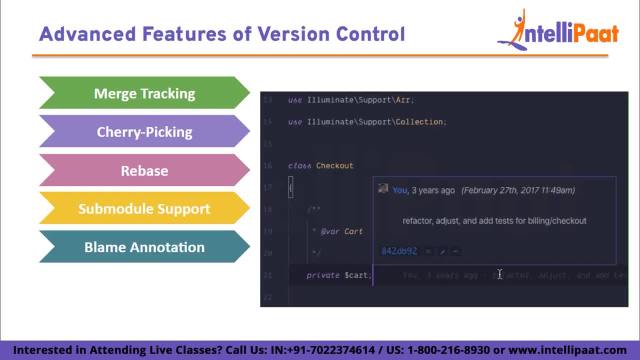 with a complex project that has multiple components. Blamannotation. blamannotation is also known as file annotation or annotation view. show who made the changes to the file and when. It allows you to view the commit details and authorship for each line of code, providing the value insights into the history or the 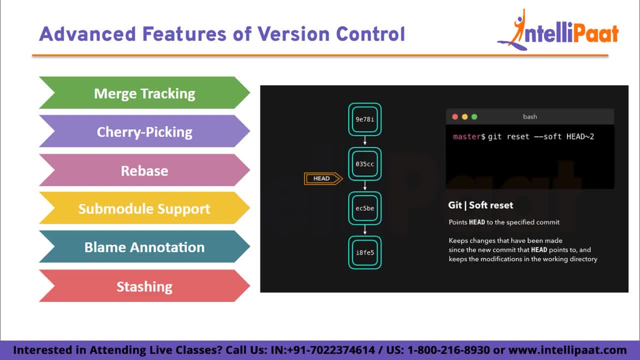 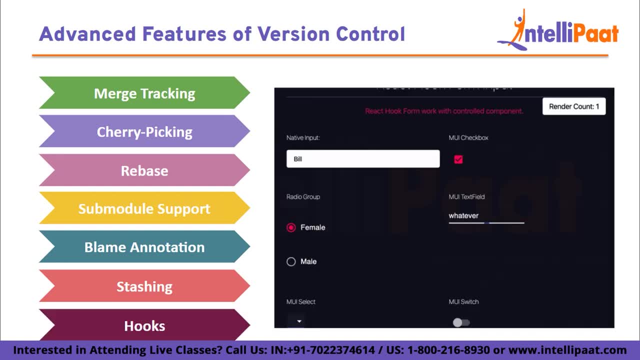 ownership of the code segment. Stashing. Stashing is a feature that allows you to temporarily save changes that you do not have to commit immediately. Hooks- Hooks are the scripts that can be triggered at a specific event in the version control flow, such as pre-commit. 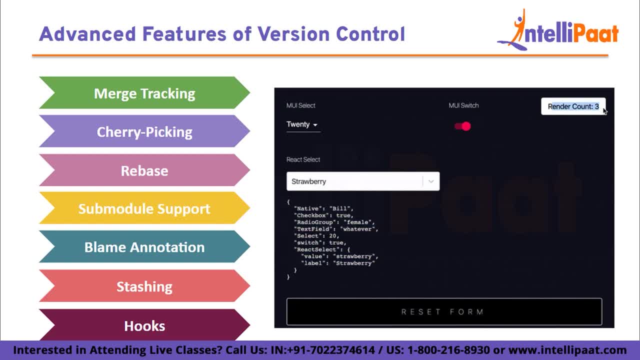 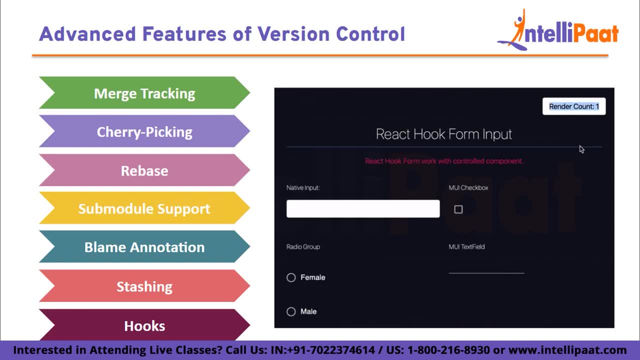 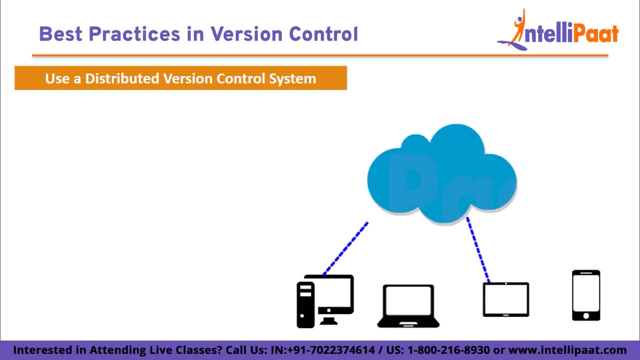 post-commit and pre-push, etc. They allow you to customize action and automate processes such as running tests, code formatting or triggering a building process, helping to enforce development best practices. So here are some of the best practices in version control. Firstly, we have User-distributed version control system. 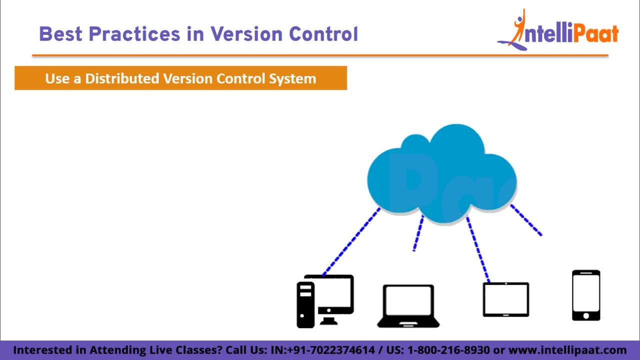 Distributed version control systems like Git offer numerous advantages over centralized systems. They provide local viewability repositories, allowing developers to work offline and commit changes locally before synchronizing with a central repository. Git is the most popular DVCS and widely used in the industry. 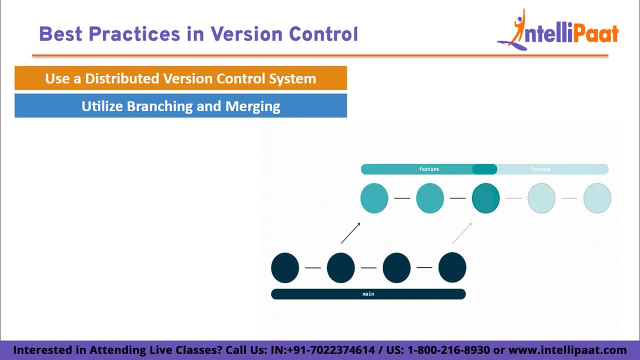 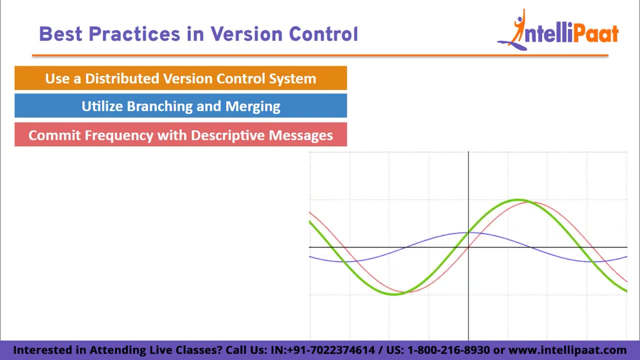 Utilize branching and merging. Branching allows parallel development of features, bug fixing and experiments. It is important to follow the branch model, such as Git flow, to keep the codebase organized. Commit frequency with descriptive message. Commit should be made frequently and clear, Concise and meaningful messages. Each commit should represent the 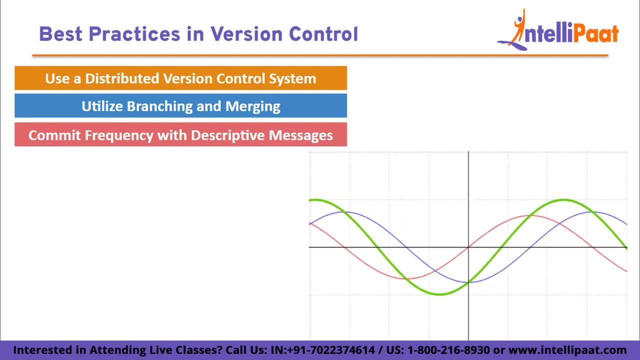 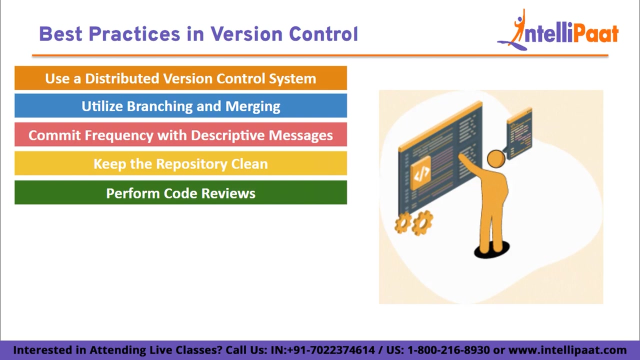 logical changes or a set of relative changes. This practice aids to understand the history of project and making it easier to revert or cherry pick specific commit if needed. Keep the repository clean. Avoid committing unnecessary files such as building artifacts, temporary files. Editor-specific settings. Perform code reviews. Code review helps to maintain the code quality. 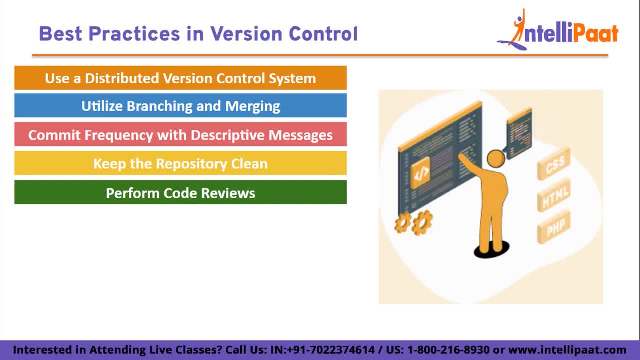 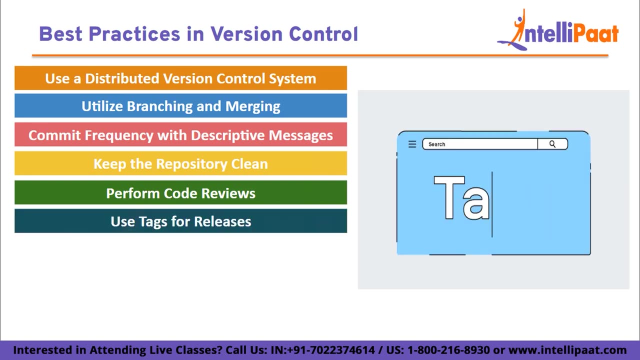 identify issues and promote the knowledge sharing within the team. Full request or similar mechanism facilitating the review process. Reviewers should focus on the code readability, best practices, adhering the code standards and portable bugs or vulnerability. Use tags for release Tags are labels assigned to specific. 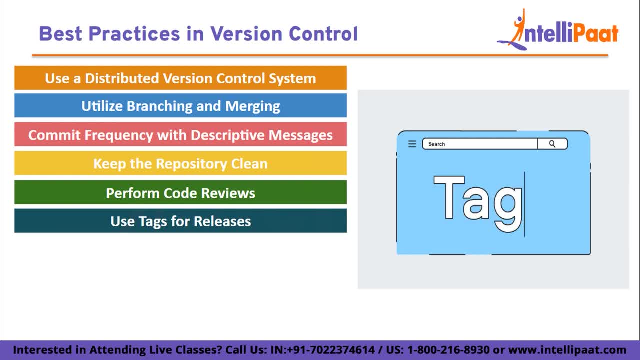 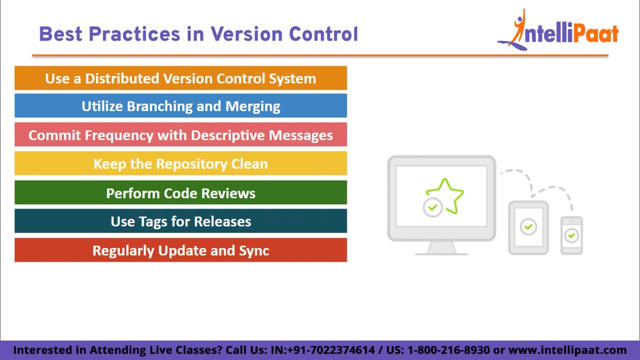 commits typically used to mark the important points in development, such as release or major milestone. Applying tags allow each navigation through the project history and provides references for stable version. Regularly update and sync, Search and pull the changes from the central repository regularly to stay updated with. 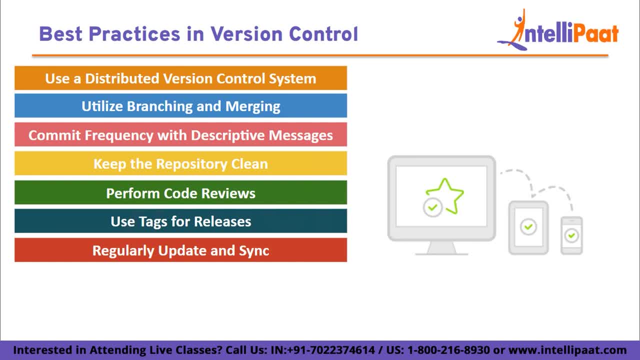 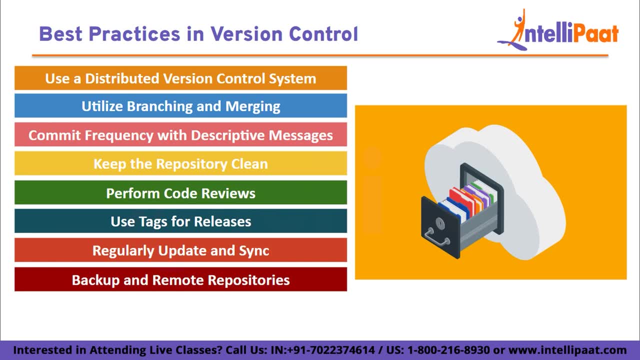 the latest changes made to the other team member. Syncing frequently helps to prevent the merge conflict and ensures a smooth collaboration process. Backup-and-remote repositories: Always keep backups of your repositories to prevent the data loss. moet Additionally consider setting-up remote repositories as a backup and to facilitate some team collaboration. 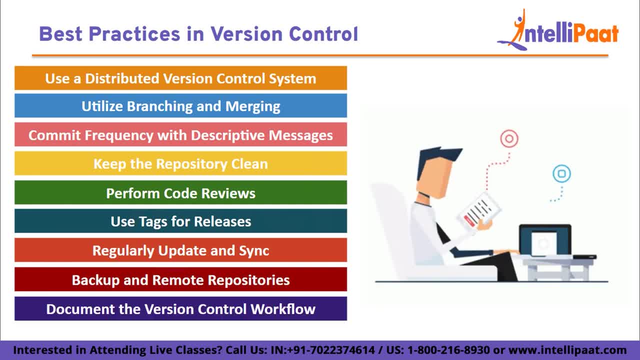 especially for distributed teams. Document the version control flow. Joinka culturally, NIGD- the most advanced разр psychologically notion, is being added on install menu. Create a documentation or README file outlining the version control workflow adapted by the team. Include instruction for setting-up the repository branching guideline committing. 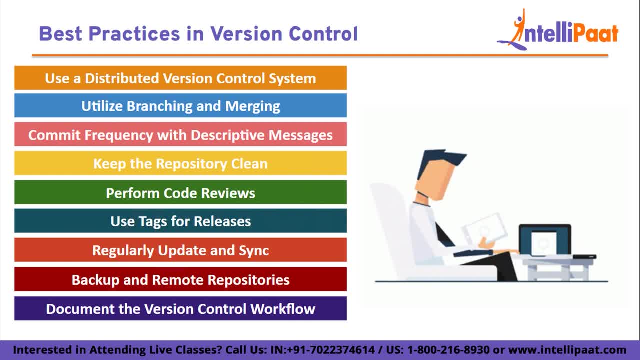 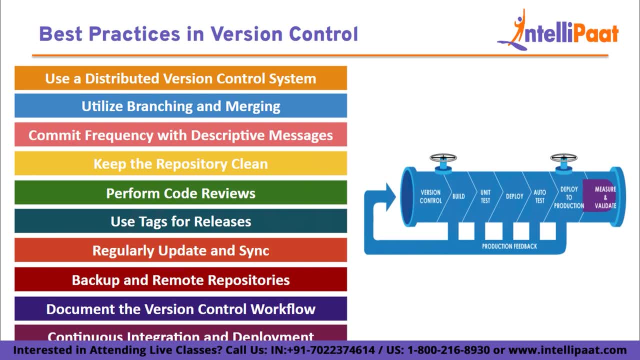 and specific convention or policies followed by the team. Continuous integration and deployment: Integrate version control with CI or CD pipeline to automate building, testing and deploying software. CI CD ensures the changes are thoroughly tested and deployed reliably, reducing the changes of introducing error in the production environment. 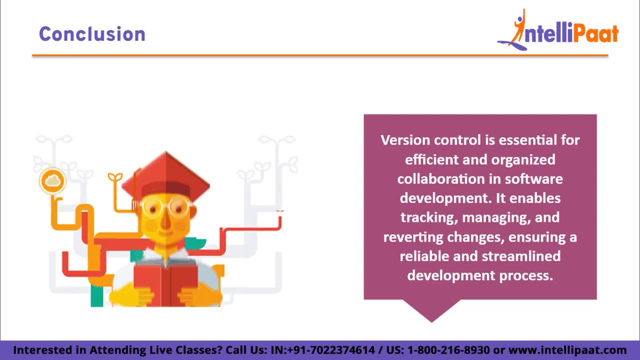 Conclusion: Version control is a critical and an indispensable tool for modern software development team. By utilizing a distributed version control system like Git, and following the best practices, developers can efficiently track the changes, collaborate seamlessly and maintain the code quality. Branching and merging strategies enable the parallel development. 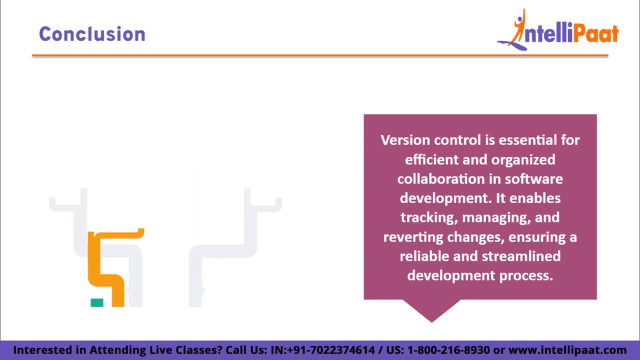 and organize code base. While frequently commit with the descriptive message, provides a clear insight into the project evolution. Code reviews foster collaboration, ensuring the higher code quality and knowledge sharing. Employing tags for releasing and regular synchronization with the central repository keeps the history organized and up to date.